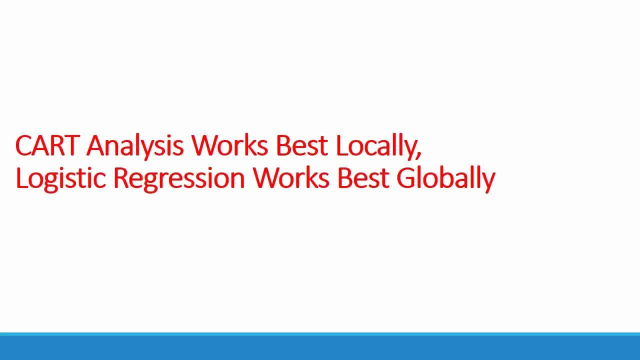 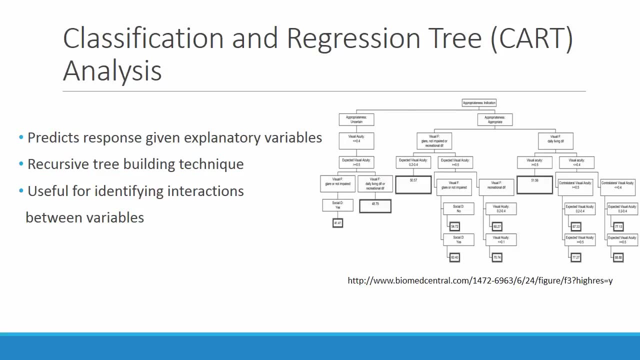 Logistic regression, on the other hand, was able to do that much more easily. Before we explain our analysis, we will first give you an overview of CART analysis. CART analysis, or categorical and regression tree, is a recursive tree-building technique that is used to identify interactions between explanatory variables. 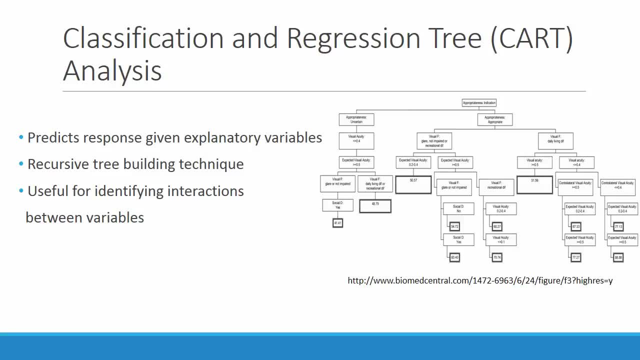 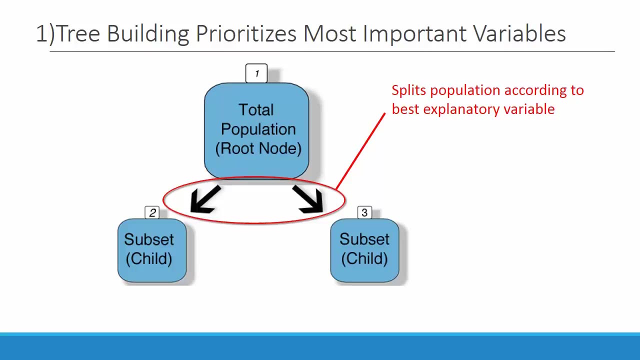 There are four main components: tree-building, tree-stopping, pruning and testing. And to understand CART, it is essential to understand the following: CART analysis begins with the process known as tree-building. To begin constructing the tree, we would begin with a root node that contains the entire population of the dataset. 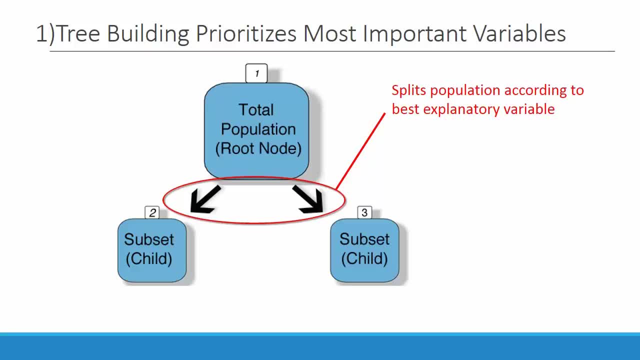 Within this population. the CART software checks all of the possible splitting variables using a Gini or Tuing splitting function. These functions then identify the best splitting variable and partition the population into two child nodes From each of these child nodes. this process, then, is called a tree-building. 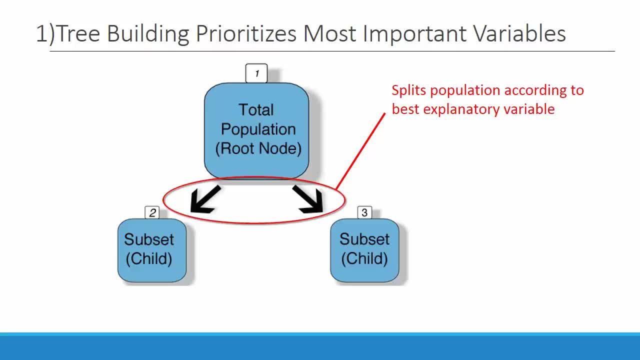 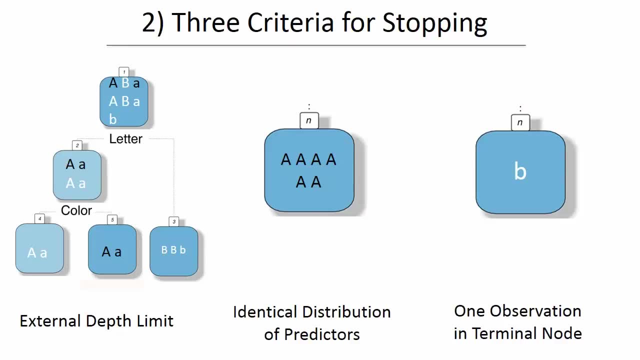 CART analysis begins with the process known as tree-building. The tree-building process then continues for each successive child node until stopping. Since the tree-building process cannot continue indefinitely, we must impose three stopping criteria. First, we can impose an external depth limit that specifies a certain number of partitions of the set. 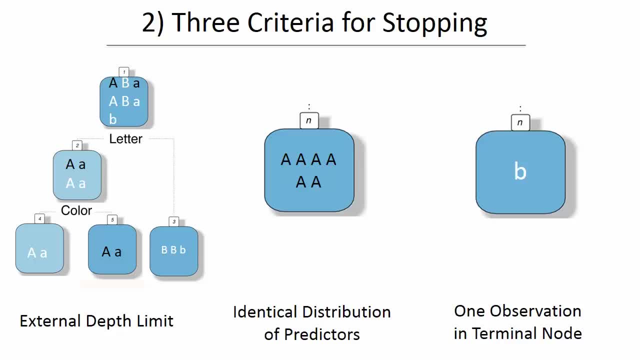 In the example below we have set a limit of two. Notice that after the first two partitions we could still split the variables by case, but this would exceed our depth restriction. The second stopping criteria is identical. We want to have a logical distribution of predictor variables. 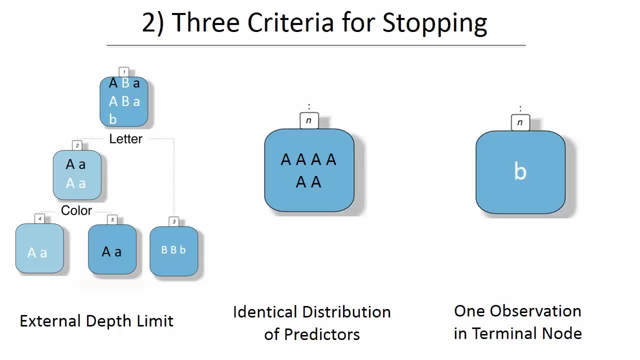 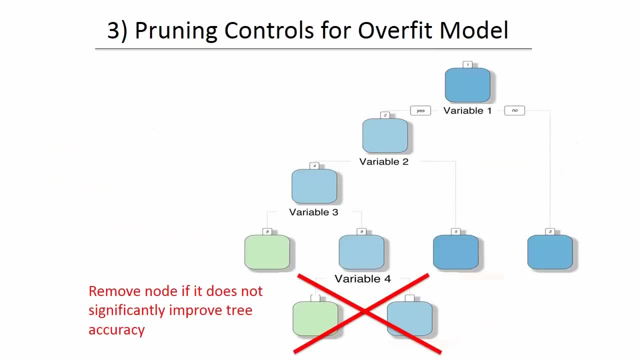 In our example here, we notice that we cannot separate this group any further. Lastly, if we only have one observation in a node, we cannot split the data any further. Unfortunately, once CART meets its stopping requirements, the resulting model is likely to be over-fit. 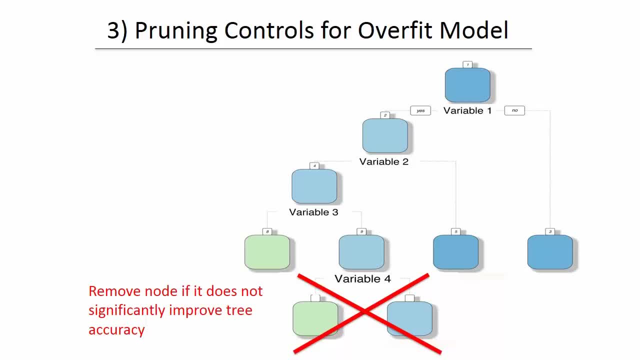 because it too closely follows the nuances of the original dataset. In order to make the CART analysis more robust, we must cut down or prune the tree. to make it simpler, We do this by using a cost-complexity pruning model that begins at the terminal node and seeks to balance the complexity of the tree with the accuracy of the prediction. 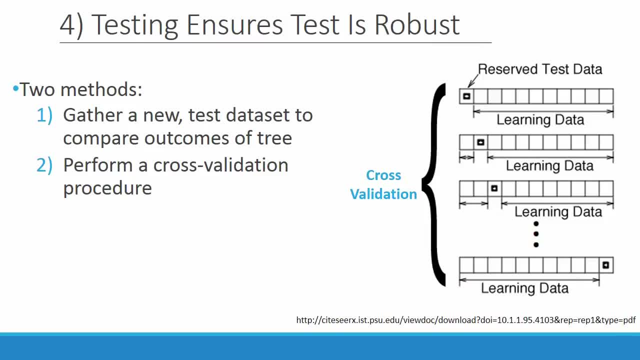 To assure the robustness of our model, we must then test the dataset in one of two different ways. First, we can test the model against an entirely new dataset and determine how accurately our previous model predicts the outcomes of the new population. This new dataset, however, is often hard to come by or costly to produce, so we can also check the model internally by performing a cross-validation procedure. 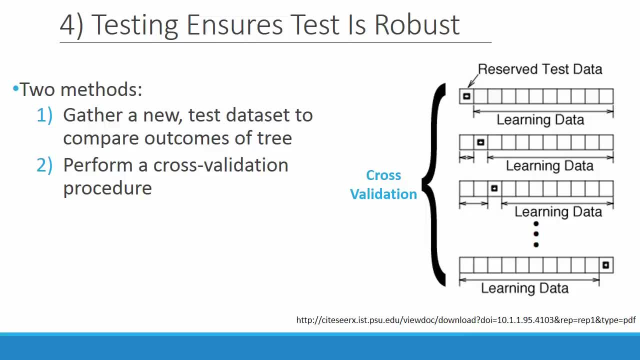 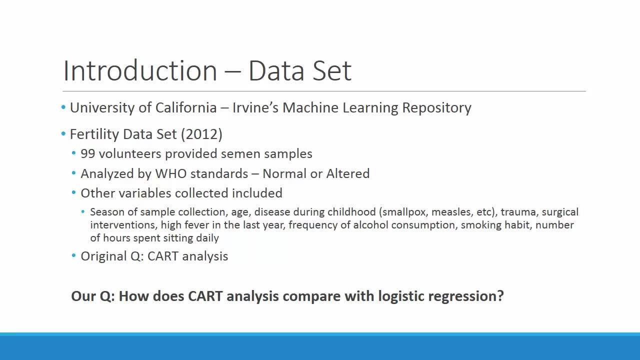 The cross-validation procedure splits the test population into N distinct subgroups and uses each individual group to test against the remaining N-1 groups. The average performance of these N models turns out to be an excellent predictor of the original model's performance. We found our dataset on UCI's machine learning repository. 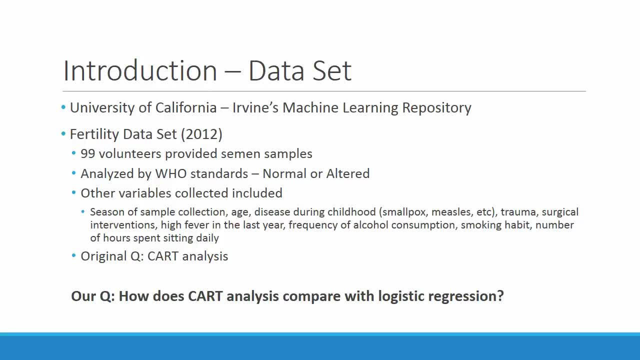 where we saw that the test population was less than 1% of the original model's performance. We also found that the test population was less than 1% of the original model's performance. The data set also provided other variables, such as the season during which a sample was collected, the age of the subject, if they had any diseases during childhood, if they experienced any trauma and if they had surgical interventions, as well as if they had high fever during the last year, and the frequency of their alcohol and smoking habits and, finally, how many hours a day they needed to drink. The data set also provided other variables, such as the season during which a sample was collected, the age of the subject, if they had any diseases during childhood, if they had high fever during the last year, and the frequency of their alcohol and smoking habits and, finally, how many hours a day they needed to drink. 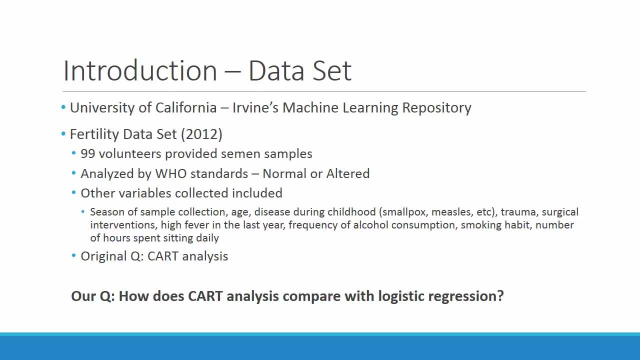 The original program sought to use these articles to predict extreme rates via cart analysis, And we were inspired to do a comparison, running our own cart analyses on the data set and comparing the decision tree that came from it with the remodels produced by running logistic regression. 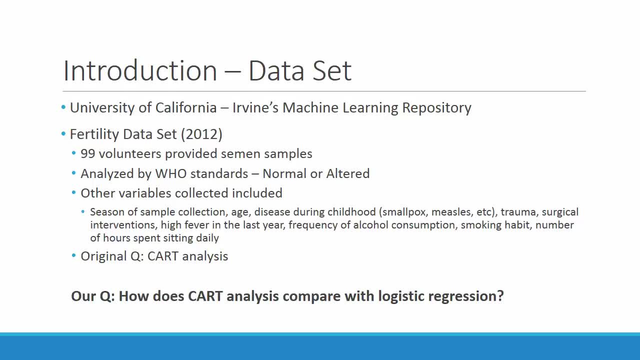 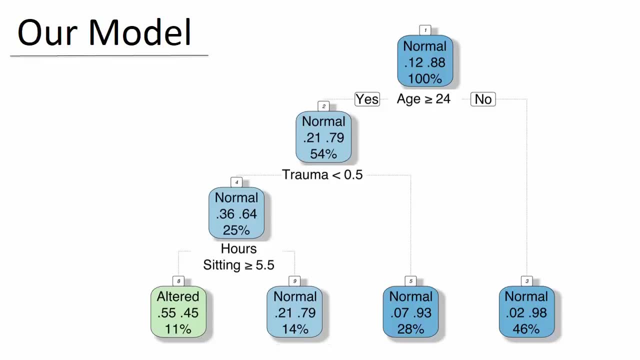 In the following slides we will be encountering our models. Here is the cart model that was produced with a data set To interpret the tree. we begin at the first node. Notice that each node corresponds to one of two levels of a response variable. 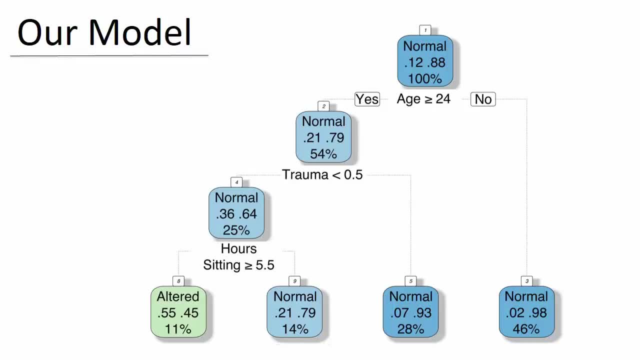 normal or altered. The middle two decimals in each node represent the percentage of individuals in each node that are correctly classified, and the bottom percentage is percentage of original population. The first node, for example, contains 100% of the population and classifies them all as normal. 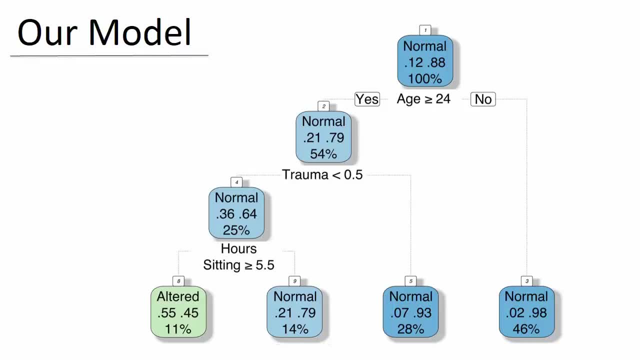 This is, of course, wrong, because we have individuals with altered semen samples in our population. so our middle two decimals take this into account, by telling us that we have incorrectly identified 12% of the samples in this node. We see, then, that the CART identifies three variables- age, trauma and hours sitting- as the best predictors for a normal or altered semen sample. 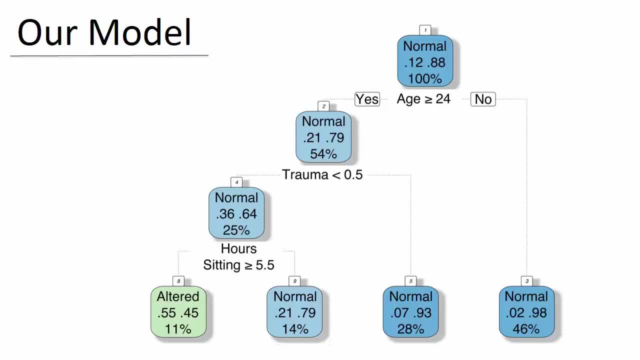 and the data did a pretty good job of predicting these outcomes, with 88% of the samples being concordant pairs. Note that the trauma variable works slightly counter-intuitively, Based on our model, if you have had some sort of trauma and are over the age of 24,. 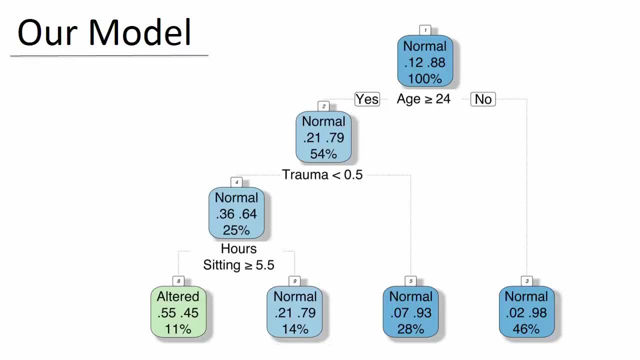 you are likely to have a normal semen sample. This runs counter-intuitively. We will now move on to the results for our logistic regression and could be results for our inability to test our model on a different data set. We will further discuss the limitations of our analysis in the conclusion section. 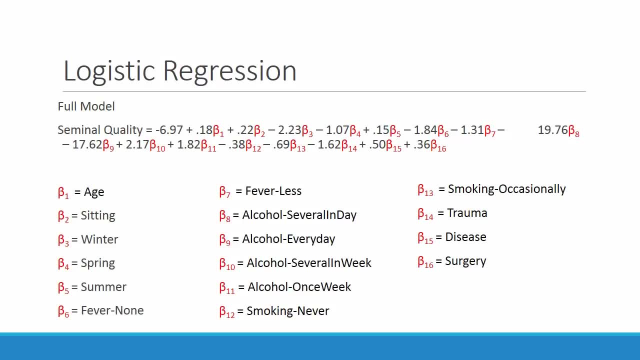 So now that we have seen our CART analysis, we can then look at the logistic regression portion of our comparison To find the most parsimonious model. we first ran a logistic regression on all the variables to determine which were worth performing drop and deviance tests on. 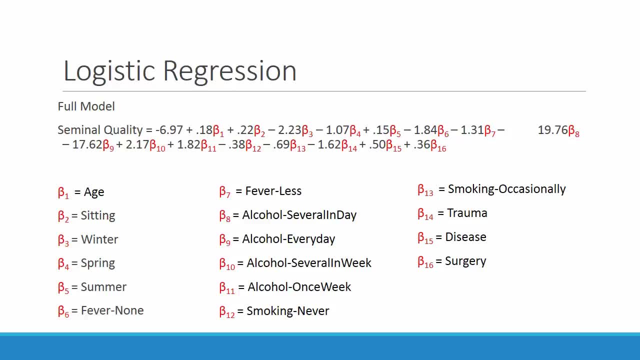 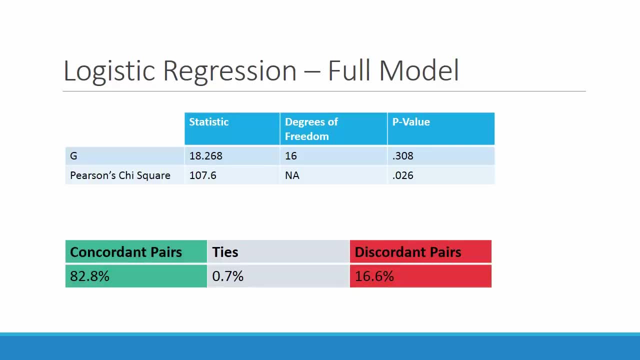 This was our full model and, as you can see, it involves many variables, and all of these variables are very similar. Although the p-values are not shown, not many were significant. As you can see on this slide, the full model has a fairly high G-score and the p-value was insignificant. 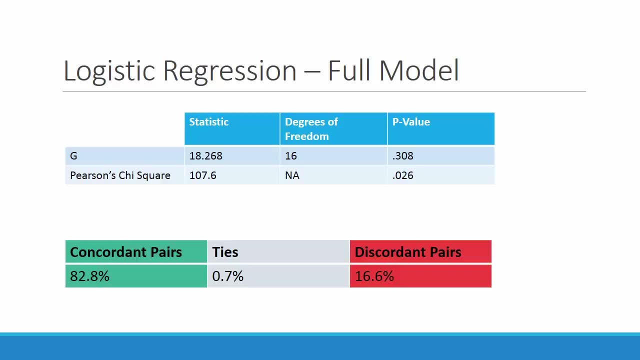 We are further concerned about this model, seeing as the Pearson's chi-square deals with a significant p-value, meaning that the model had a poor fit. However, as we note the concordant and discordant pairs, this model actually has a pretty high percentage of successful predictions. 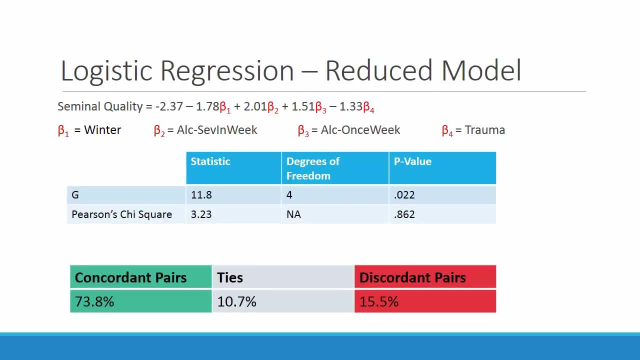 As we continue to find a more parsimonious model which has a more comparable variable count to that of the CART model, we conducted many drop and deviance tests. Finally, we arrived at this logistic regression model, which has four variables that were significant or very close to significance. 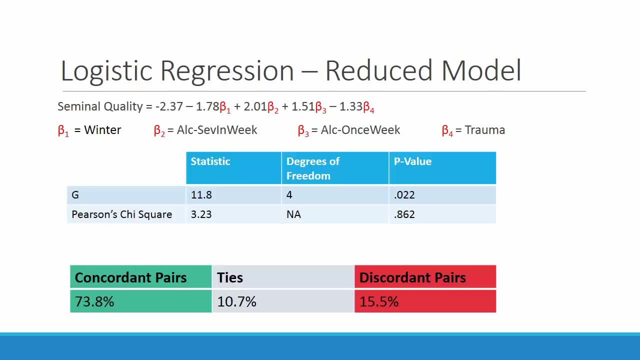 This model has a p-value of 0.022, as well as a Pearson chi-square p-value of 0.862,, which suggests that this has a good fit. However, as you can see, the percentage of concordant pairs decreased from the previous full model's 82.8% to a 73.8%. 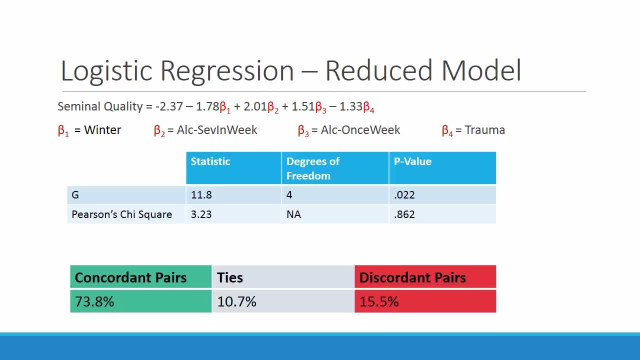 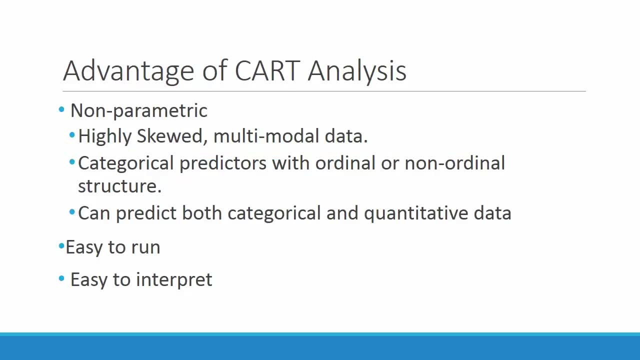 although it is important to keep in mind that this was a trade-off of having a good fit. There are many advantages to using CART analysis, the most useful one being its ability to handle non-parametric data. This allows us to conduct analysis on highly skewed, multi-modal data sets and not have to check if the model assumptions are being met. 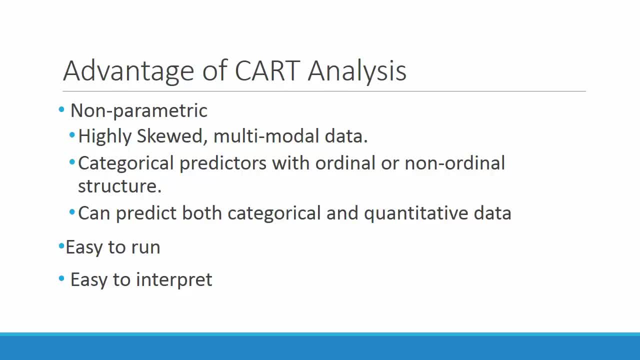 CART analysis can also be used to analyze both quantitative as well as categorical data, whereas logistic regression can only handle categorical data and linear regression can only handle quantitative data. Therefore, using CART analysis saves a lot of time and is useful for conducting analysis on large, messy data sets. 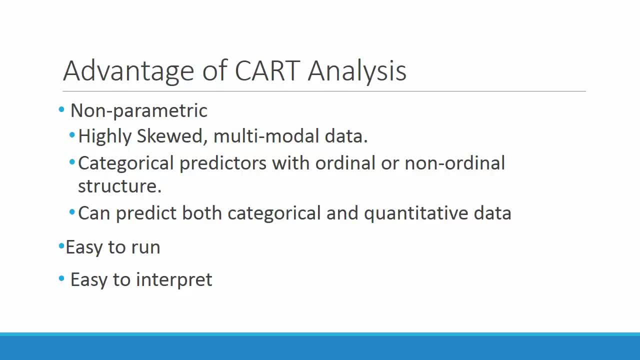 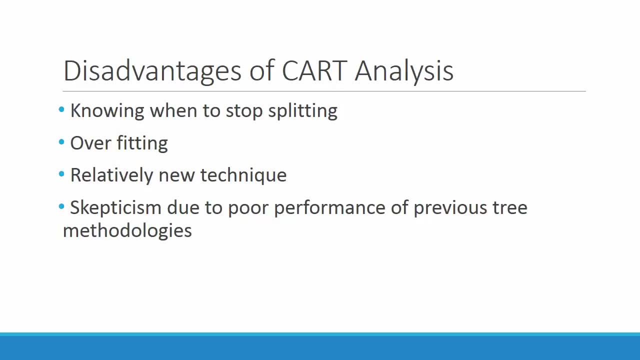 CART analysis is also easy to run and easy to interpret, making it a very useful technique when trying to communicate results to non-statisticians. One problem to watch out for when using CART analysis is overfitting the data, Since it is hard to know when it is appropriate to stop splitting a tree. 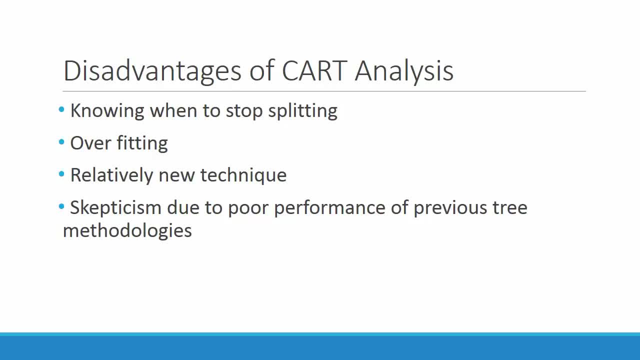 it might be tempting to add additional nodes to make the model more precise. This, however, makes the analysis less robust, as this analysis will then be tailored to the specific data set being used. Statisticians are also hesitant when they use CART analysis due to how new the technique is. 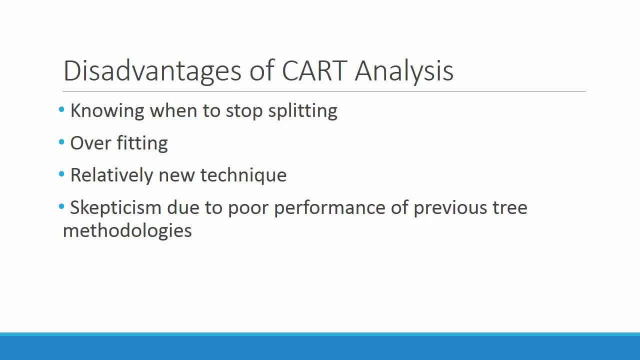 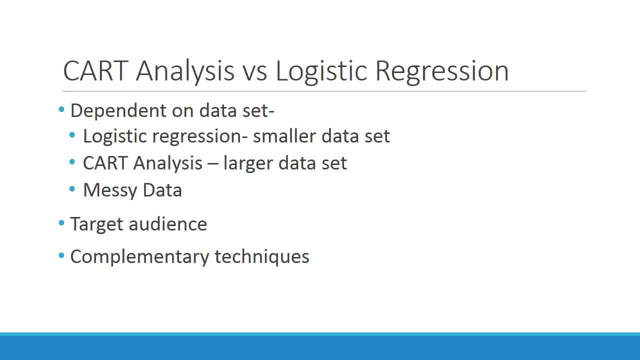 and due to the poor performance of previous tree-based methodologies. Therefore, when trying to decide between using logistic regression and CART analysis, it may be useful to keep certain things in mind. Logistic regression is better than CART analysis when the size of the data set is small. 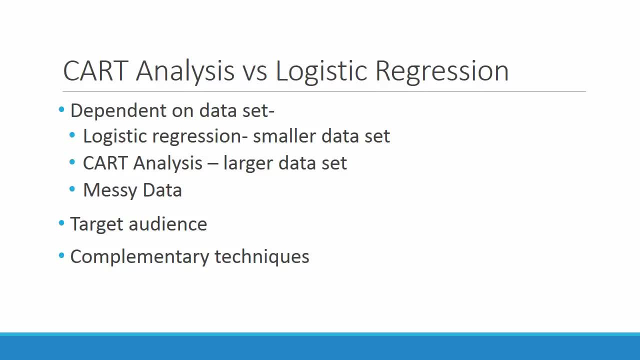 CART analysis, however, is more efficient when dealing with large, messy data sets. It may also be useful to keep in mind the audience to which the analysis is being presented to. CART analysis may be more useful when presenting results, when presenting to non-statisticians. 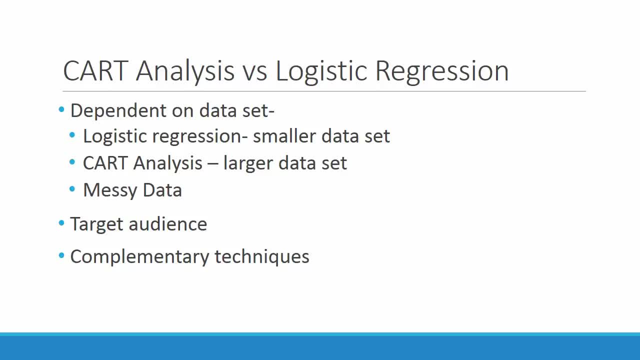 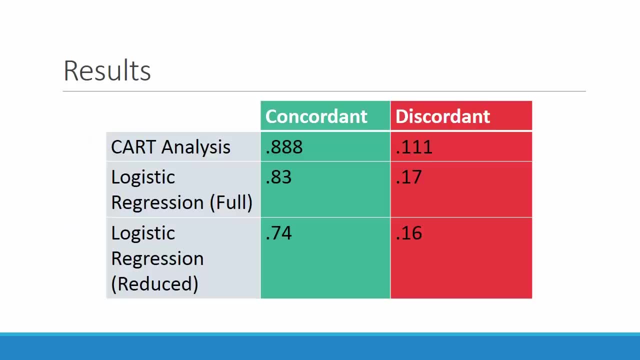 while logistic regression may be preferred when presenting to statisticians. However, both techniques are highly complementary and could be used together to conduct robust tests that are easy to communicate. We try and compare the two different techniques by looking at the number of concordant pairs in each. 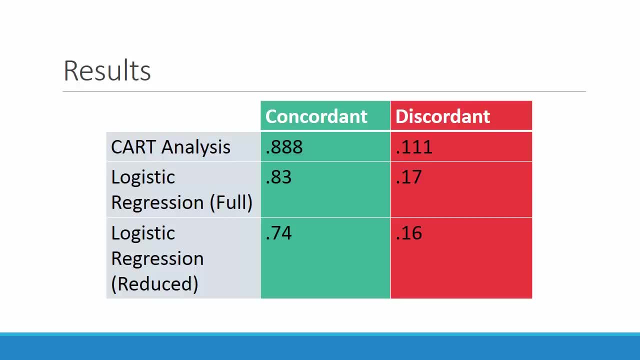 We find that the highest number of concordant pairs is in CART analysis, with 88% of the pairs being concordant. We then have the full logistic regression model, with 83% of the pairs concordant In the reduced logistic regression model.